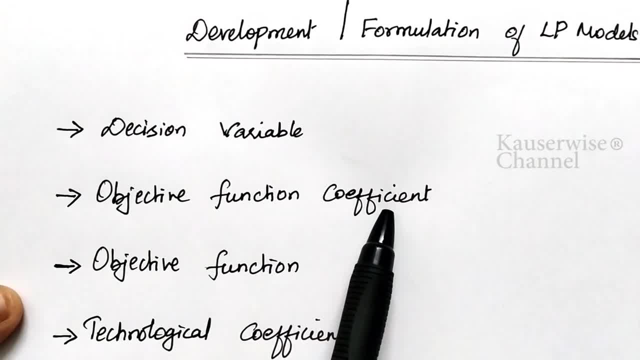 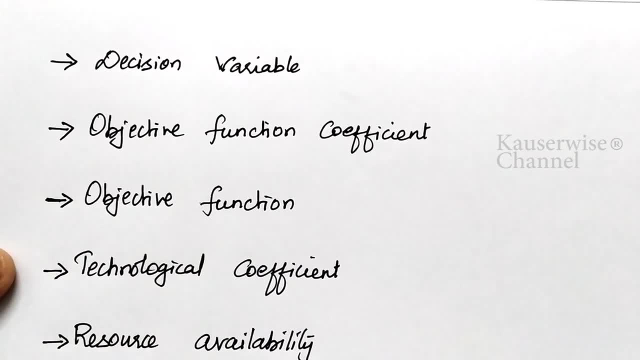 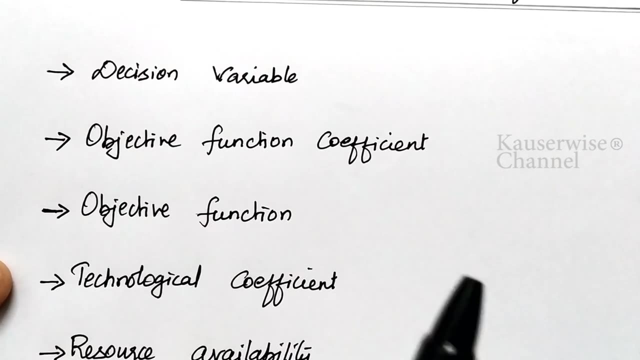 out an activity. Okay, so it is also one of the element in the LPP formation. The next one is objective function, See objective function. it's an expression representing the total profit or cost of carrying out a Set of activity at some levels. Okay, see, the objective function will be either maximization. 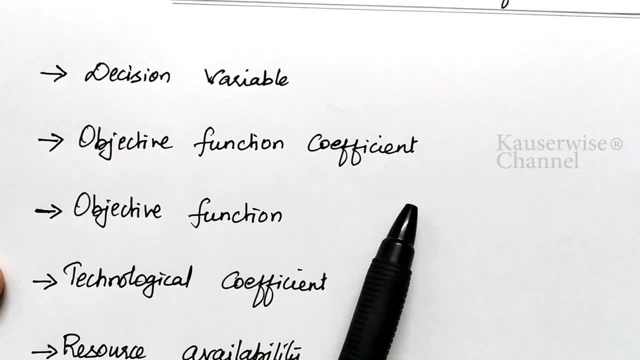 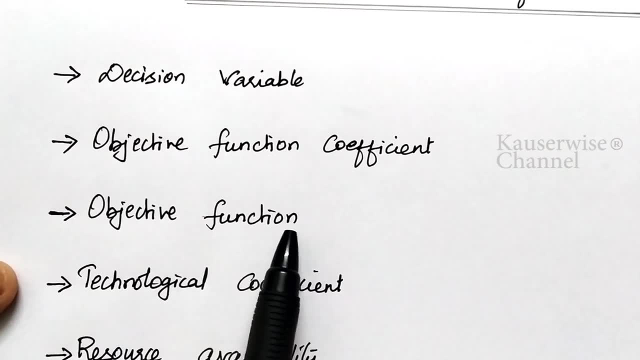 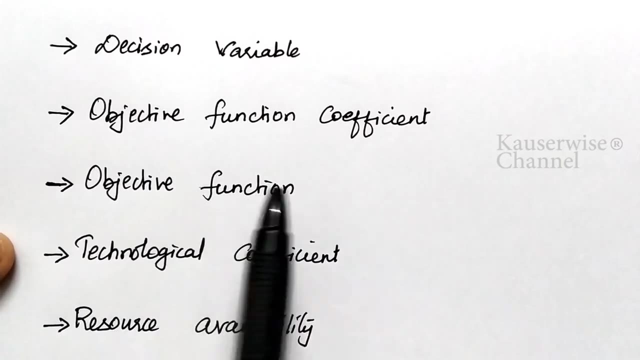 type or minimization type. If it is maximization means, our objective function will be maximizing the profit. If it is minimization means minimizingizing the cost of production, Okay, this is very important in the formation of LPP. That is objective function: either maximization or minimization. 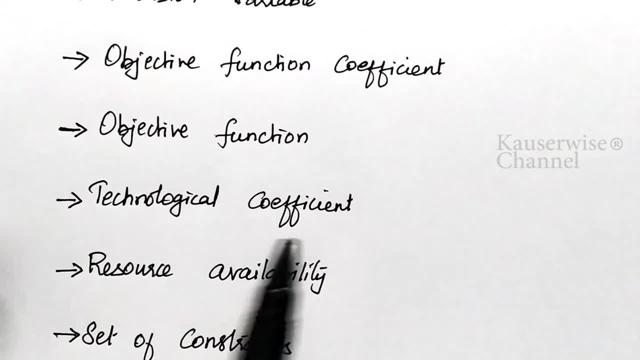 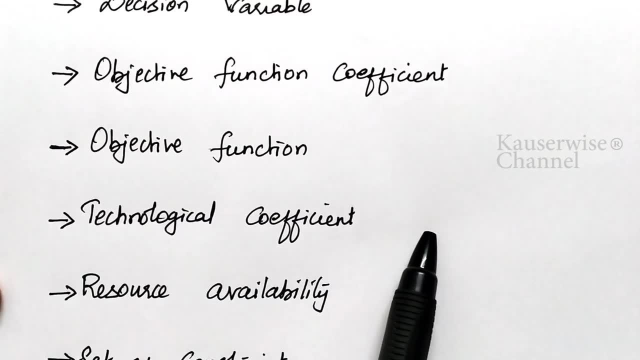 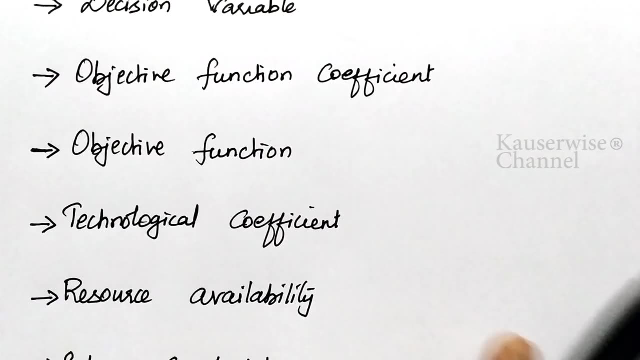 Okay. the next one is technological coefficient. So technological coefficient means here it is the amount of resources required for the activity. So, in order to complete a particular activity, what are the various resources are required to complete the activity? It's just like a matrix. Okay, this is called as technological coefficient. 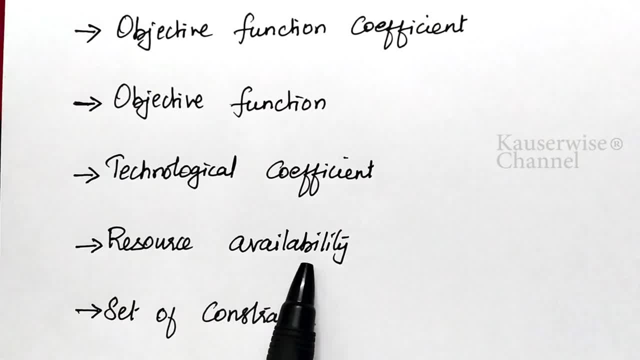 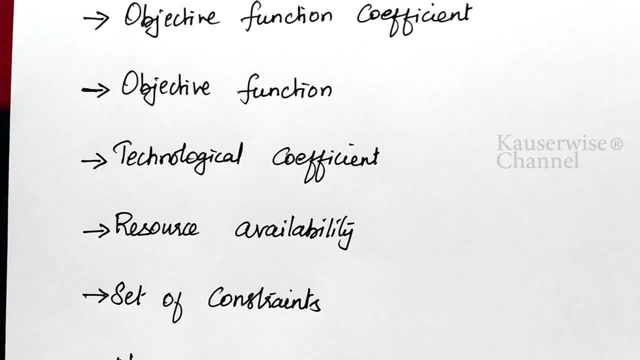 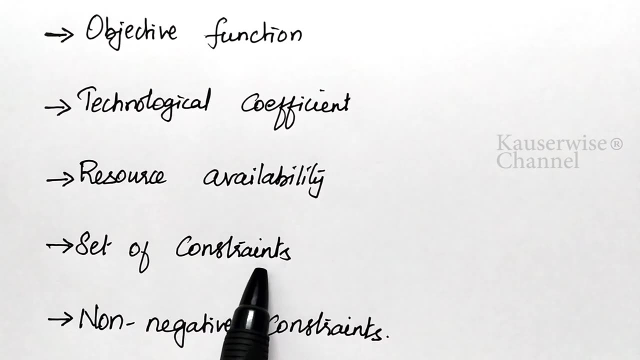 And the next one is resource availability. The resource availability means the amount of resource available during the planning period. Okay, during a particular period, What are the resources available to complete the task? It's called resource availability. The next one is set of constraints. See, a constraint is a kind of restriction on the total amount of a. 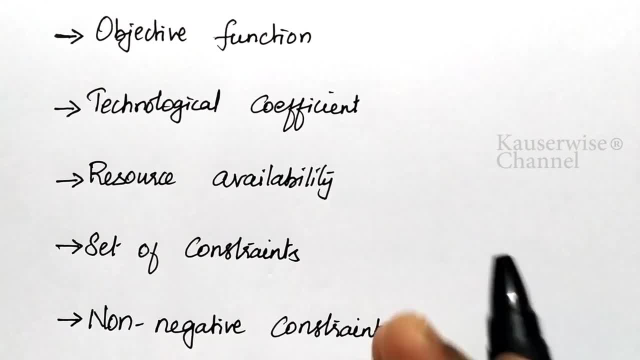 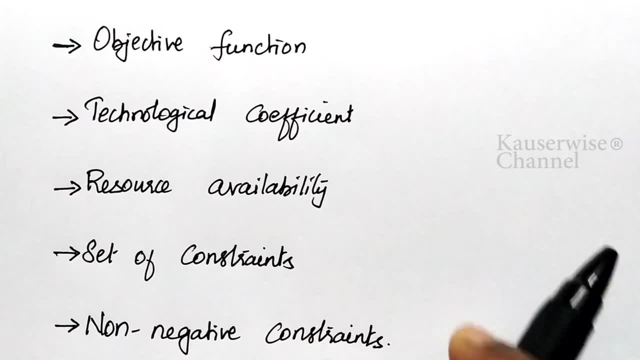 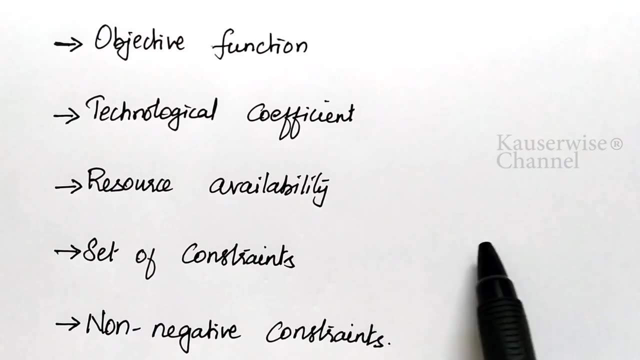 particular resource required to carry out the activities at various levels. See in the model, in the LPP model, there will be many such constraints. So these constraints will limit the levels of achievement of different decision variables. Okay, It can be lesser than or equal to, or greater than or equal to. Okay, like that. 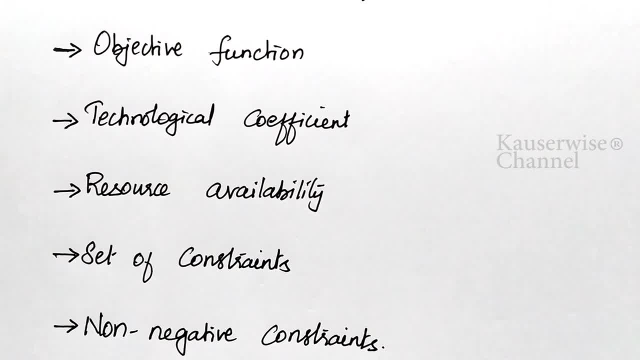 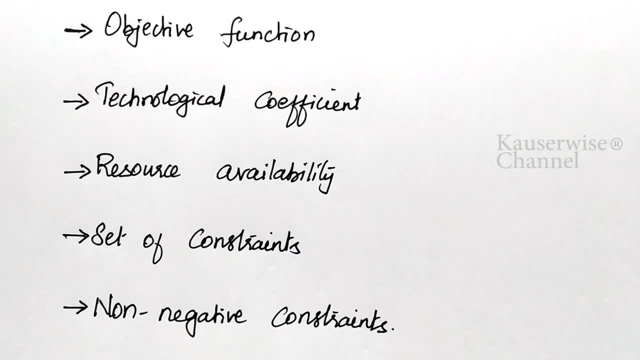 This is called a set of constraints, That is, limitations, Restrictions will be there. The last one is non-negative constraints. So non-negative constraint means positive. Each and every decision variables in the LPP model is a non-negative constraints. It should be. 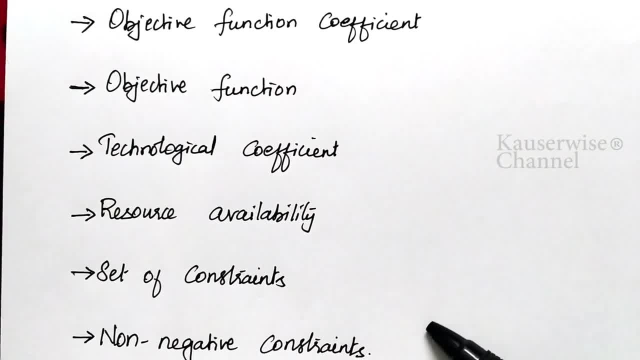 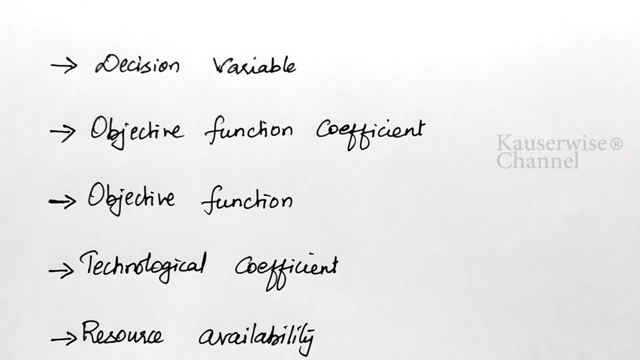 positive only. So these are the various components which is required to formulate LPP model. Now we are going to see how to formulate LPP model. Now we are going to see one problem. for better understanding, Let us see the problem. See, this is the maximization problem for development of LPP model. Okay, 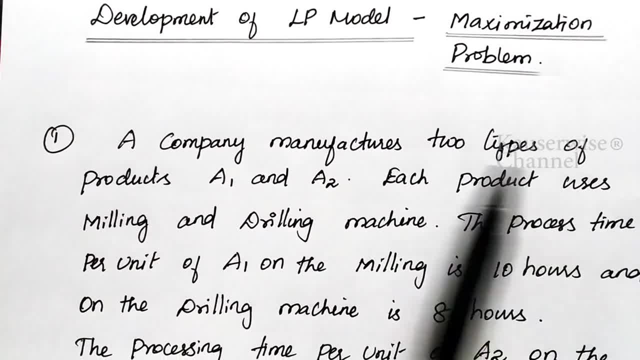 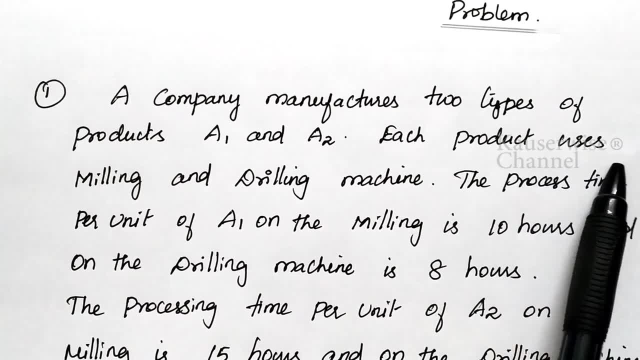 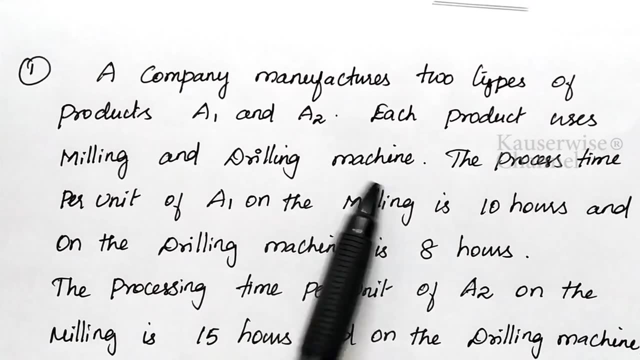 See the problem. A company manufactures two types of product, A1 and A2.. Okay, There are two different products, A1 and A2. Each product uses milling and drilling machine. So each and every product. okay, process through two different machines, milling and drilling machines. 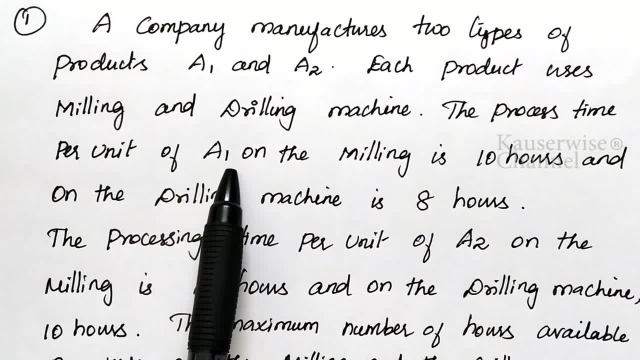 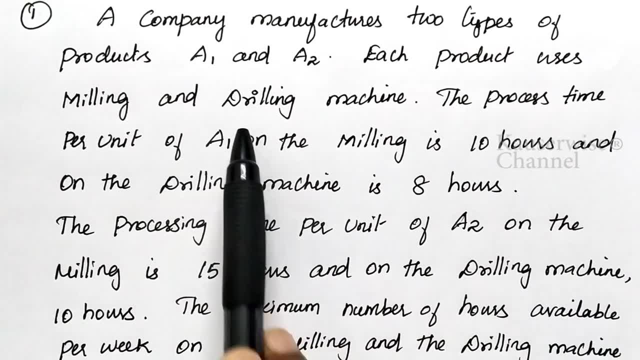 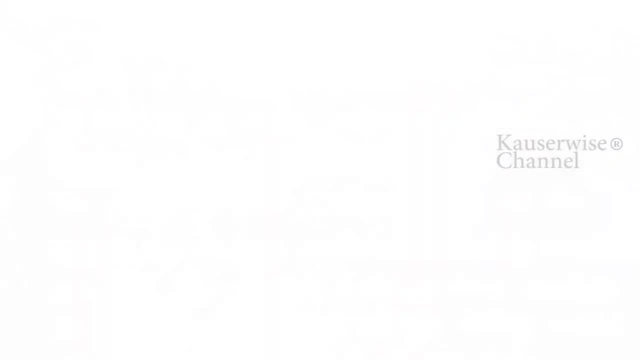 And then the process time per unit of A1 on the milling is 10 hours and on the drilling machine is 8 hours. Okay For A1 product. milling machine required for 10 hours and drilling machine is required for 8 hours. Okay To process the particular product. The processing time per: 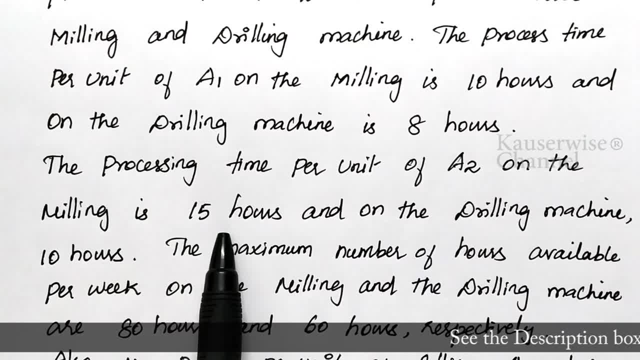 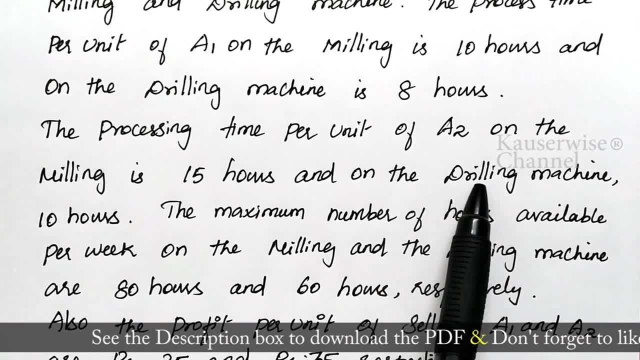 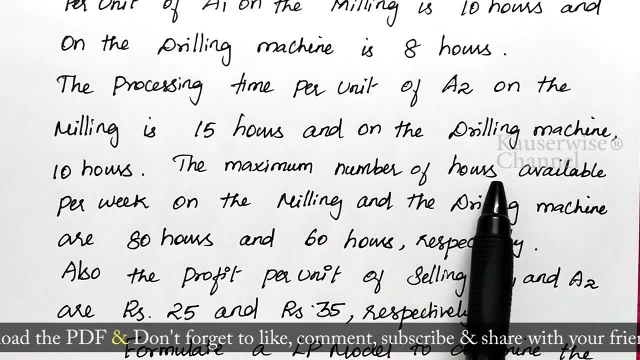 unit of A2 on the milling is 15 hours and on the drilling machine 10 hours. Okay, So A2 required milling is 15 hours and drilling Next one. The maximum number of hours available per week on the milling and drilling machines are: 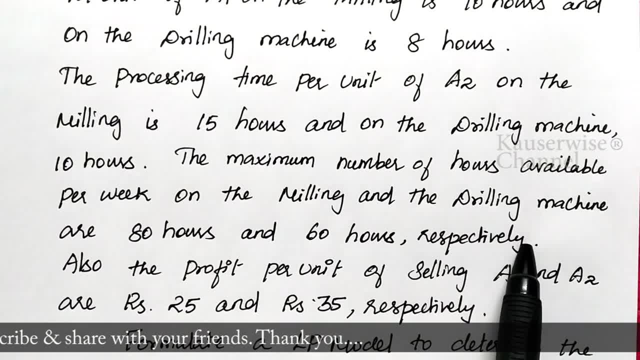 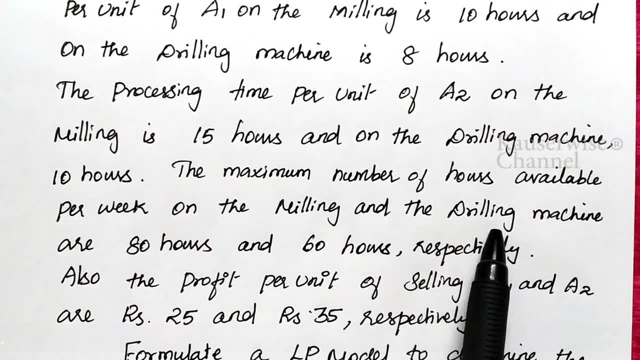 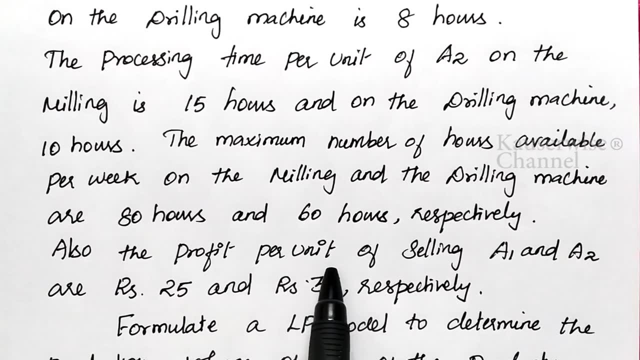 80 hours and 60 hours respectively. Okay, Per week. the maximum number of hours available is: for milling machine, 80 hours. for drilling machine, 60 hours. Okay, This is the constraint Limitation, is there? Okay, Also, the profit per unit of selling. 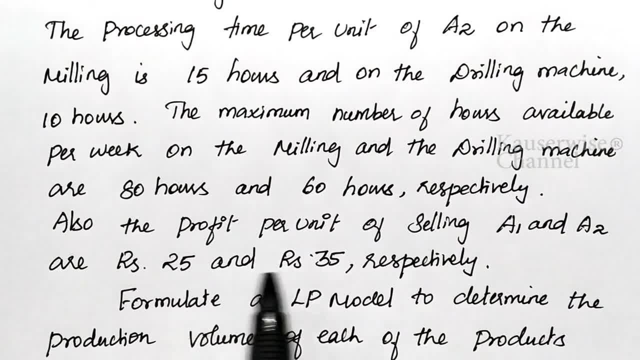 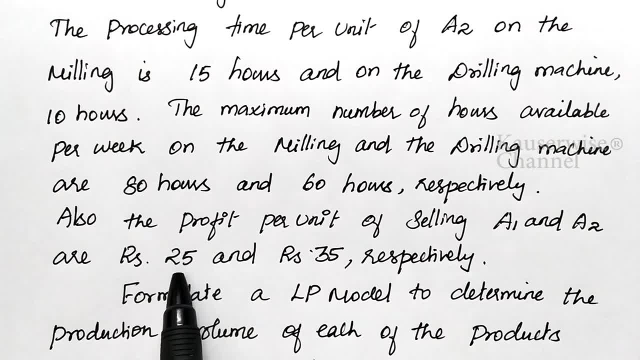 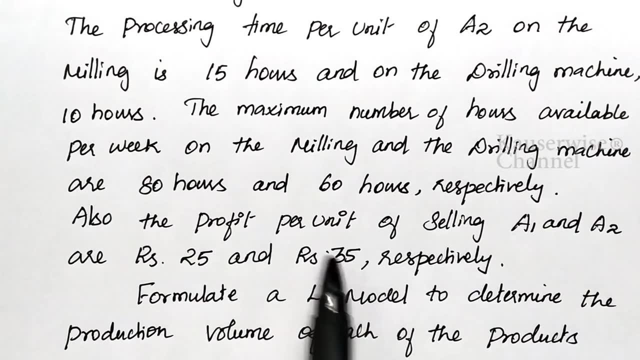 A1 and A2 are 25 rupees and 35 rupees respectively. Here profit per unit also given. For product A1: 25 rupees per unit of A1 product, Okay. And for A2 rupees, 35 rupees per unit profit. 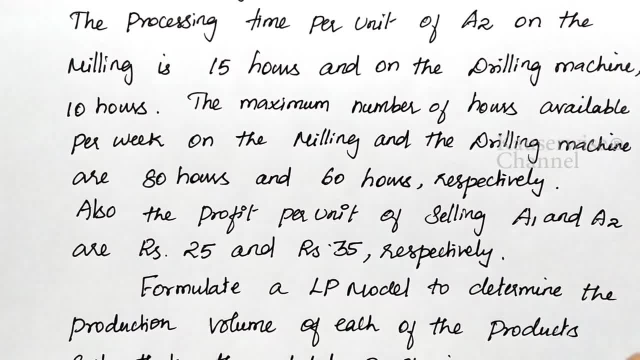 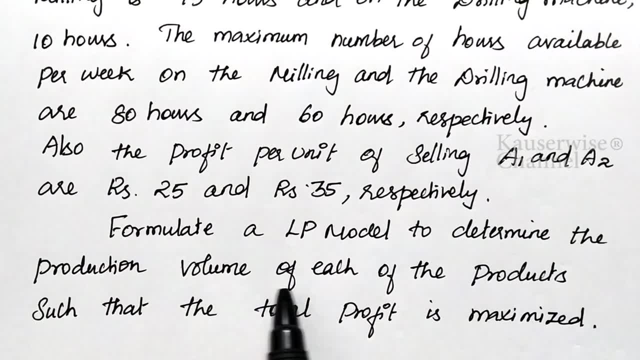 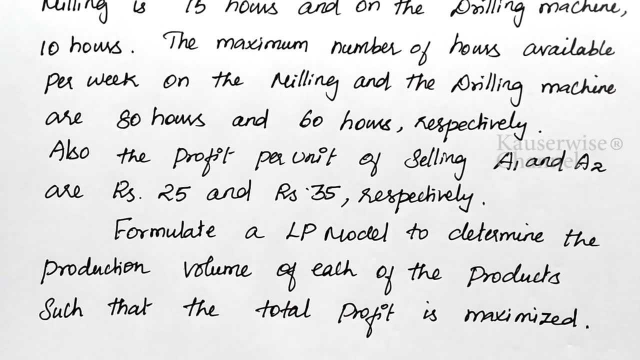 per unit. Okay, So the profit per unit also given in the problem With this information, they ask you to formulate LPP model to determine the production volume of each of the product such that the total profit is maximized. See, generally, there will be two objectives: The 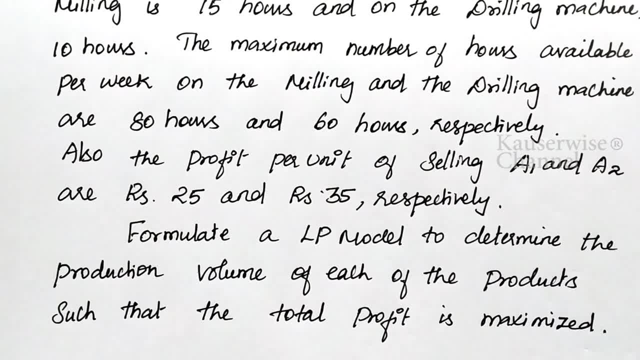 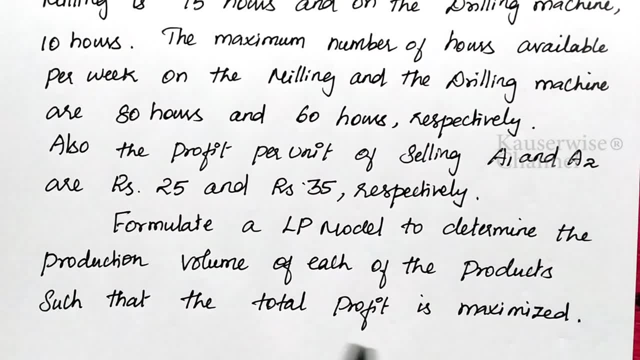 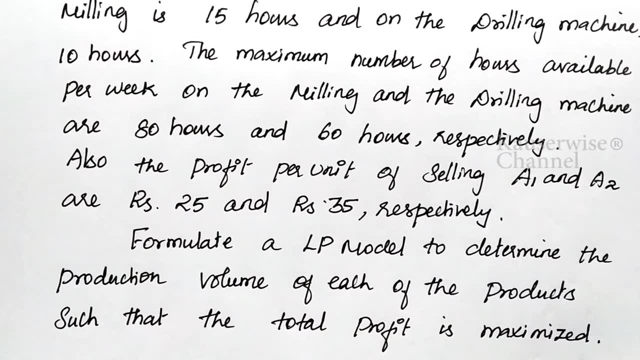 first one is maximization of profit. The another one is minimization of cost. Okay, That cost of production. But here this problem is maximization problem, That is, the total profit is going to increase. Okay, For that we are going to prepare LPP model. Now let us see the solution. See before. 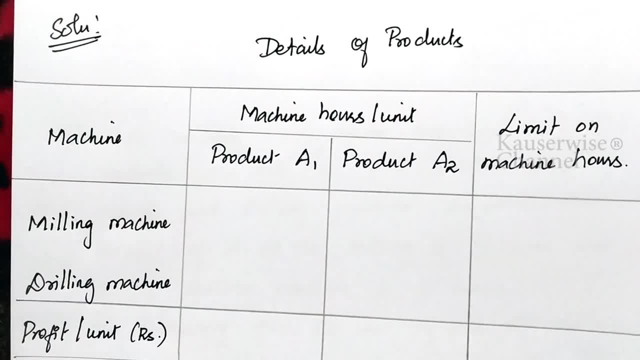 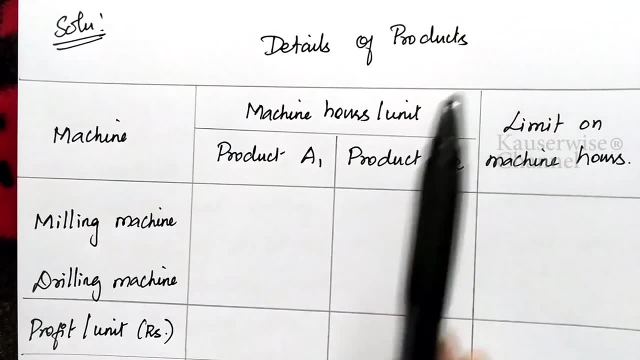 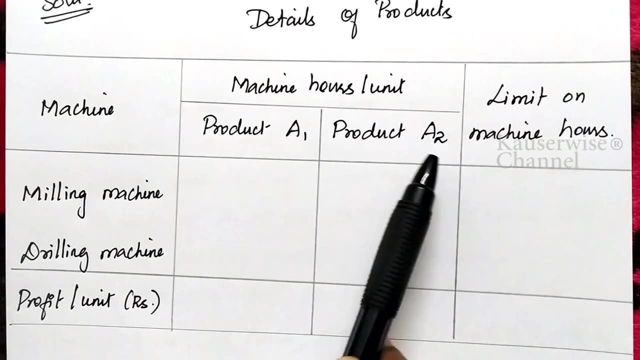 we formulate the LPP model. the first step is just prepare a tabular column based on the information given in the problem. See here details of product. Here there are two different machines, right Milling and drilling machine, And there are two products, A1 and A2.. Okay, The machine hour per unit also given in the problem, That is. 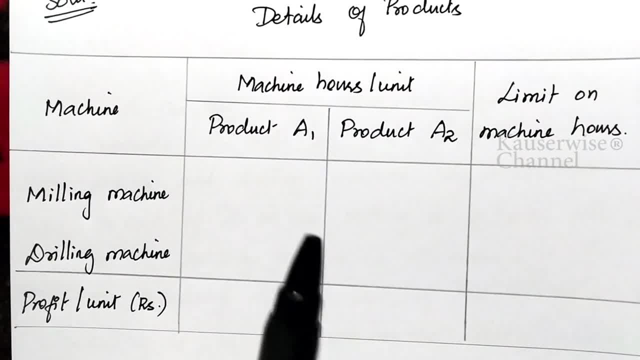 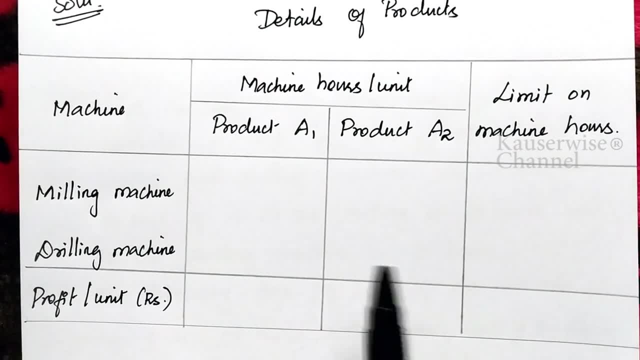 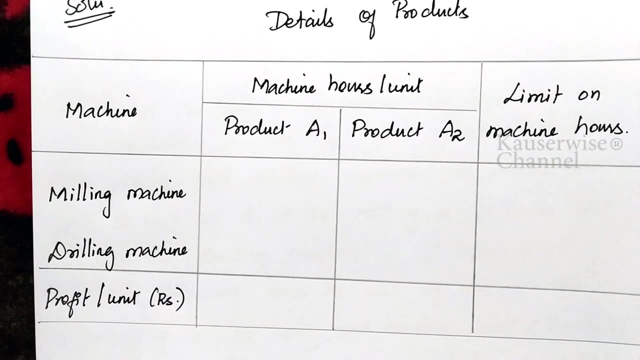 milling machine required and drilling machine required. So how many number of hours is required to produce A1 and A2.. That information also given in the problem. And the next one is limit of machine hour For each and every machine available. duration also given in the problem. Okay, 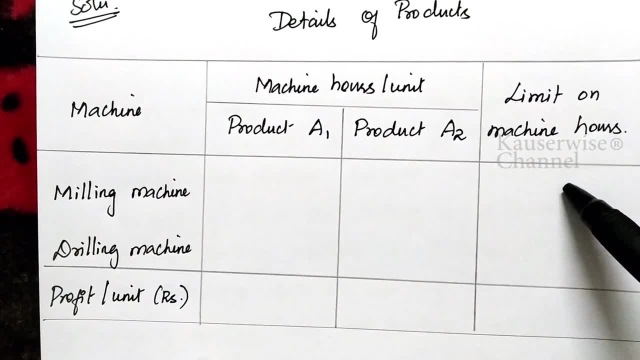 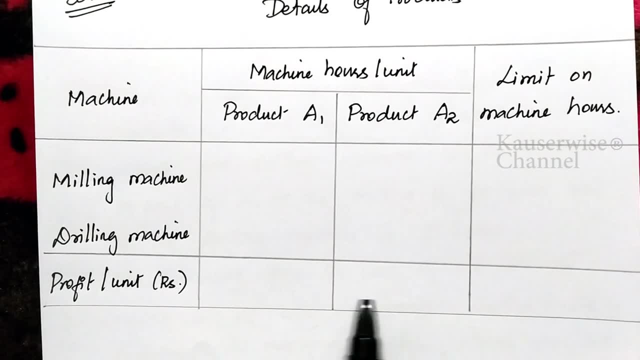 This is called as limitation, The limit on machine hour, also given in the problem, for two different machines And the finally profit per unit for product A1 and product A2, also given in the problem. So based on that first we need to construct a tabular column. With that you can. 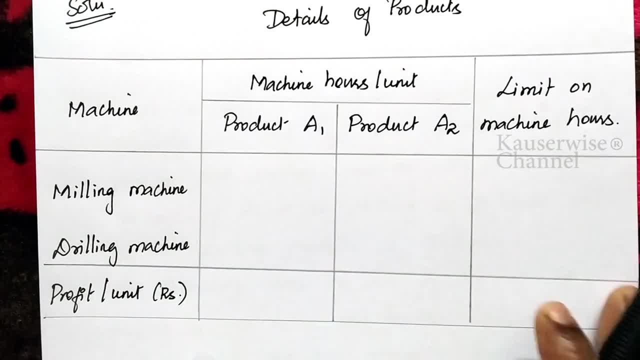 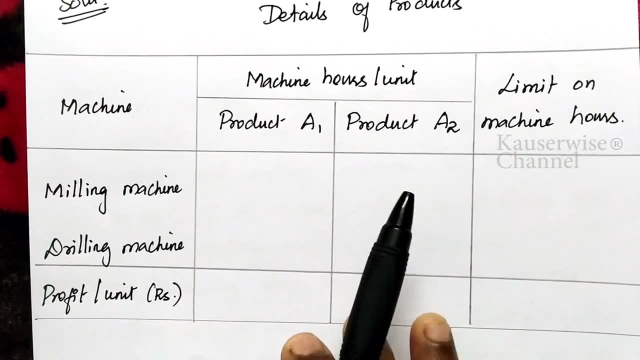 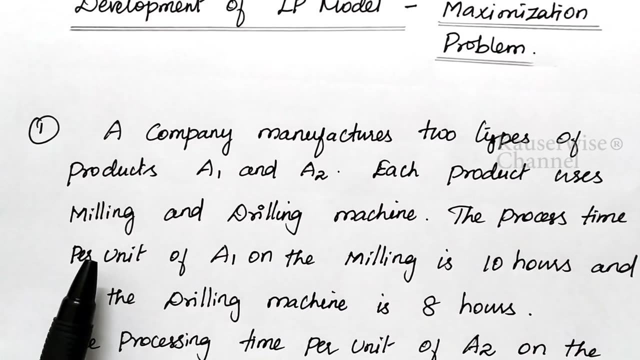 easily formulate LPP model. Okay, Let us see the information. The first one is a product A1. So how many number of machine are for milling and drilling machine? See the problem. See the problem. A company manufactures two types of product, A1 and A2.. See the tabular column. See the details of. 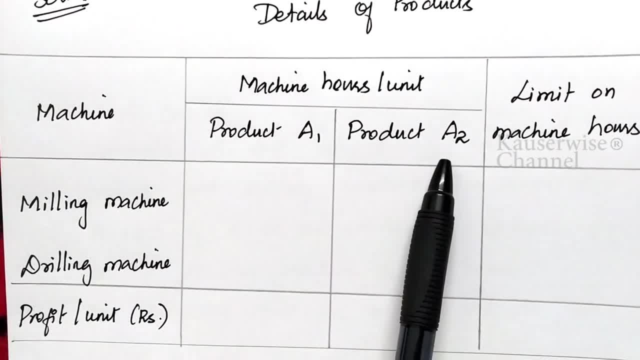 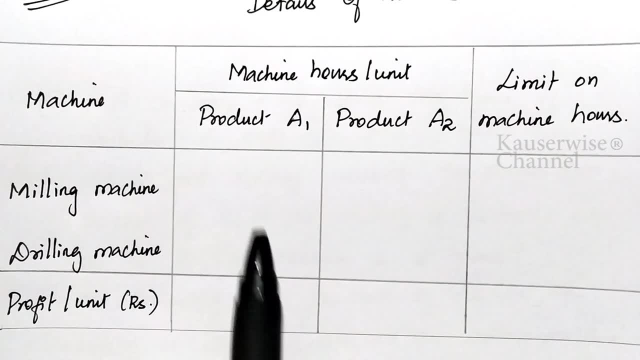 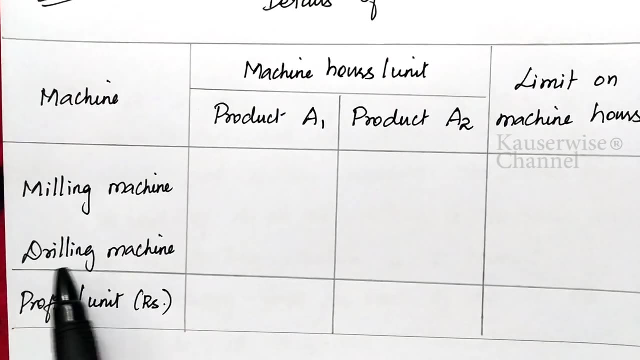 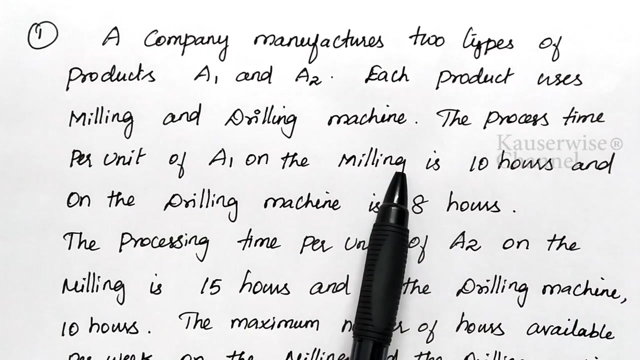 product. Here we have two different products, A1 and A2.. The next one: each product uses milling and drilling machine. Okay, See, to process A1 and A2 how many machines required? Two machines. The next one drilling machine. Okay, The next one. the process time per unit of A1 on the milling is: 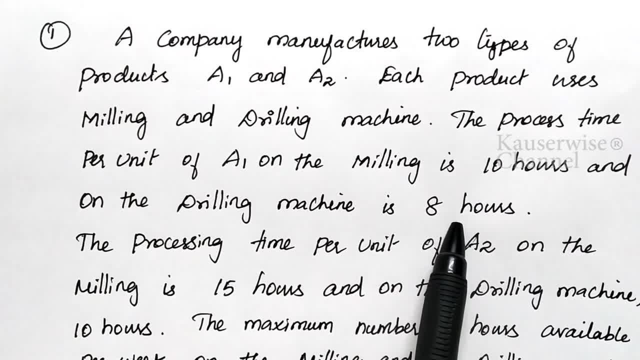 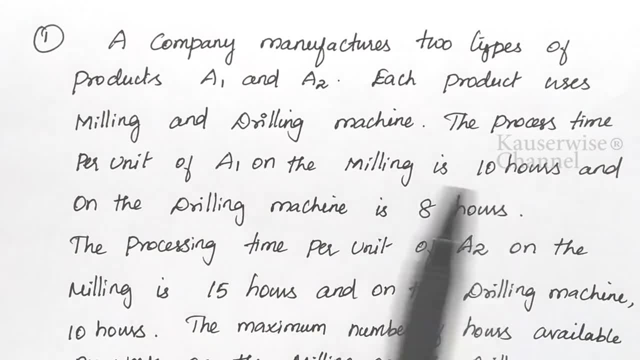 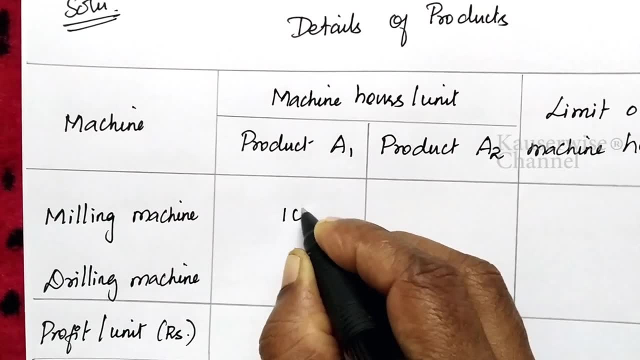 10 hours and on the drilling machine is 8 hours. Okay For particular product: for A1: how many hours for milling? 10 hours for drilling: 8 hours. Okay, See for product A1: milling machine required to process A1. for how many hours? 10 hours and drilling machine is required to process A1. how many hours. okay, And then the processing time per unit of A2. in the same way, A2 on the milling is 15 hours and on the drilling machine is 10 hours. Okay, For A2, milling machine is required for how many hours? 15 hours and drilling machine required for 10 hours. See the tabular column for product A2. 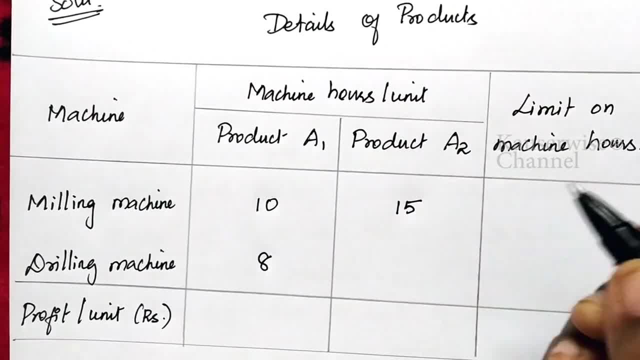 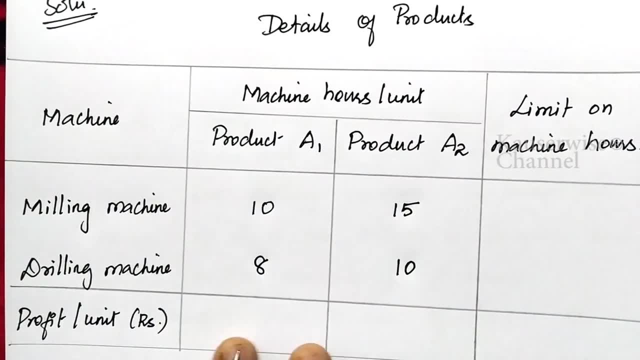 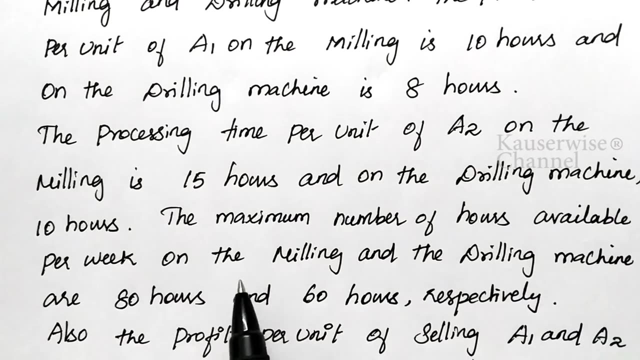 milling machine is required for how many hours? 15 hours per unit and drilling machine is required for A2 is 10 hours per unit. Okay, So this is the information given in the problem. Now see the problem. See the maximum number of hours available per week on the milling and the drilling machines. 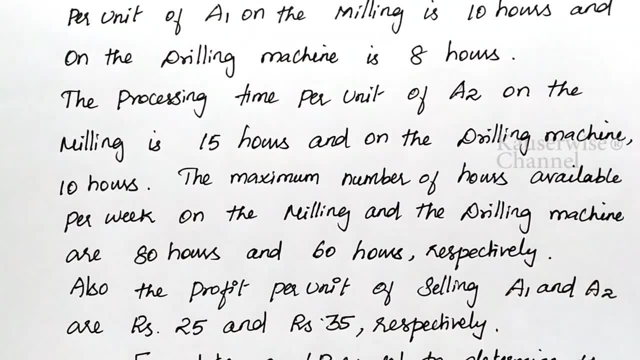 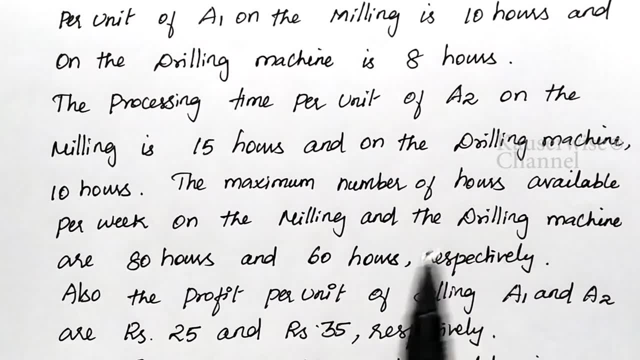 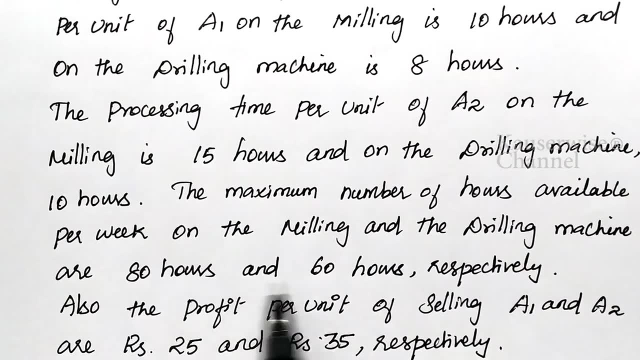 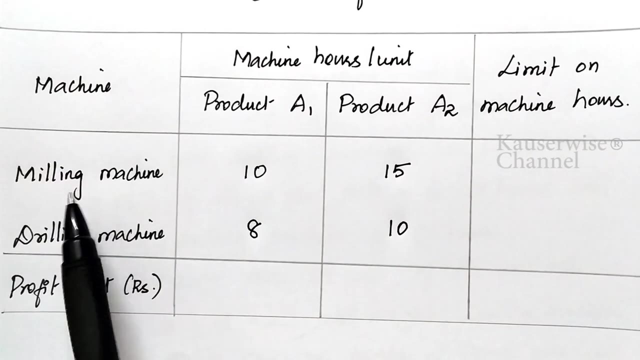 are 80 hours and 60 hours. See here the limitation is given. Okay, Milling machine. you can use it for one week. how many hours? 80 hours. and drilling machine: you can use it for how many hours? 60 hours. So this is the constraint. limitation is there? See limit on machine. are Okay Milling? 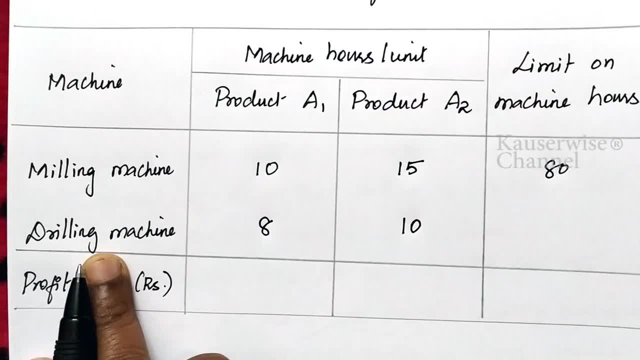 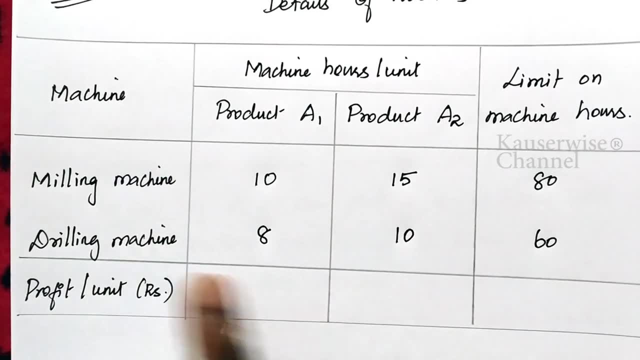 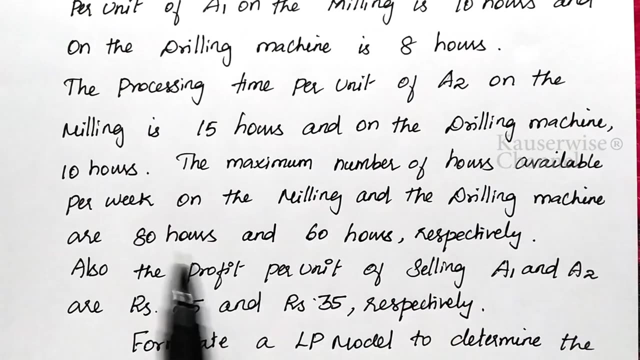 machine how many hours per week? 80 hours. and drilling machine you can use for week. how many hours? 60 hours. So this is the limitation given for milling and drilling machine. Now see the problem. See, we have entered the limit of milling machine and drilling machine per week. Okay, How? 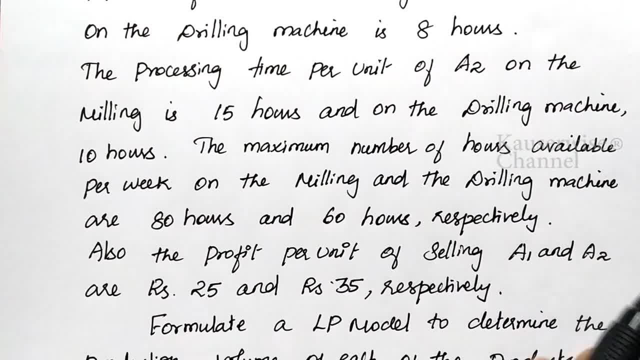 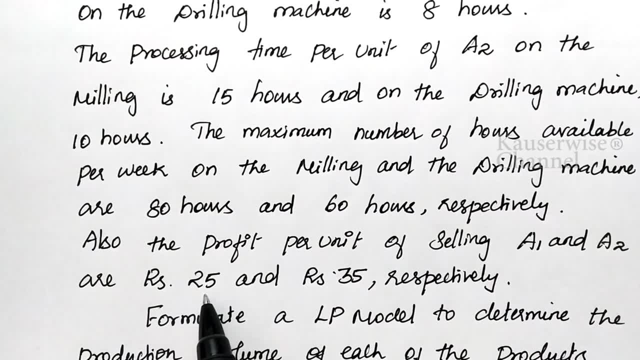 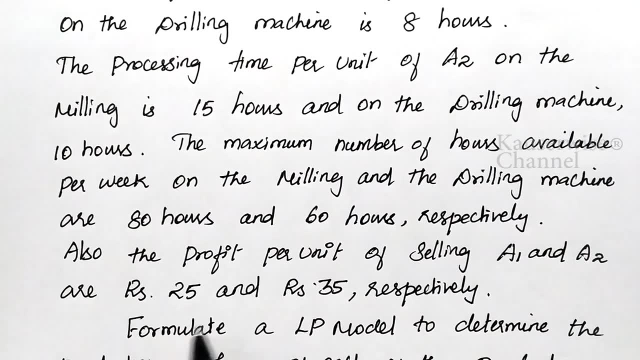 many hours: 80 hours and 60 hours respectively. Next one: also, the profit per unit of selling A1 and A2 are 25 rupees and 35 rupees respectively, Yet profit per unit of selling price of A1 and A2 also given in the problem. Okay, See the tabular. 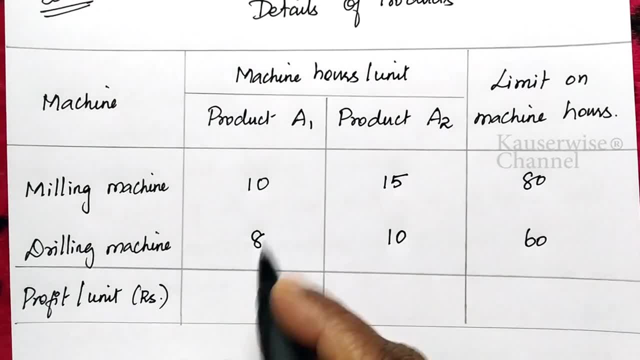 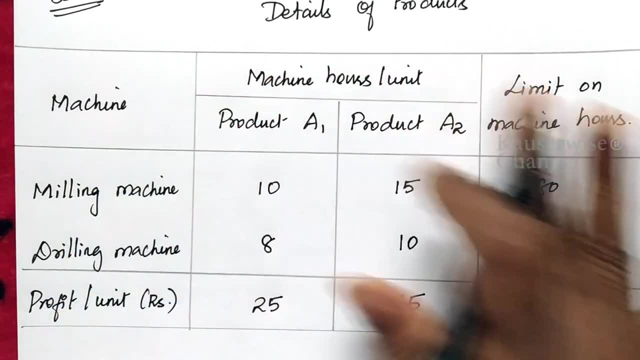 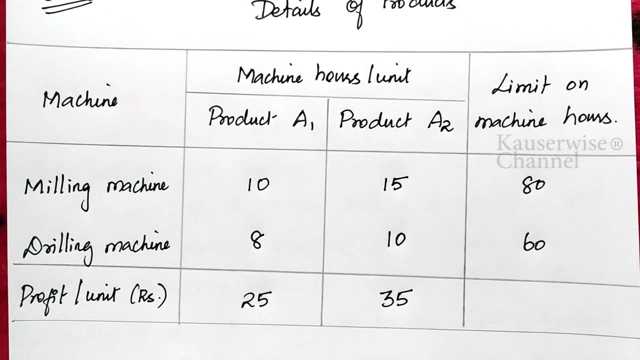 column: profit per unit for product A1 is 25 rupees per unit and for A2 35 rupees per unit. Okay, These are the informations given in the problem. So based on the information, we can easily construct the table. Okay, According to the 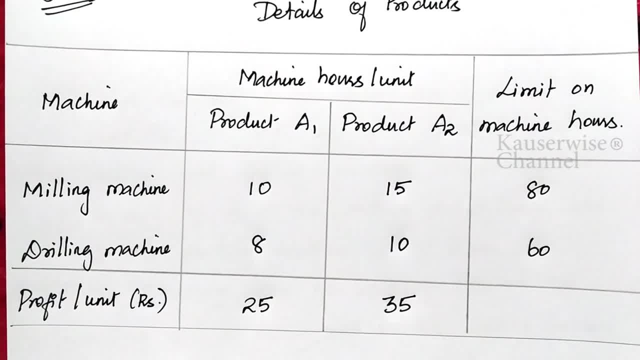 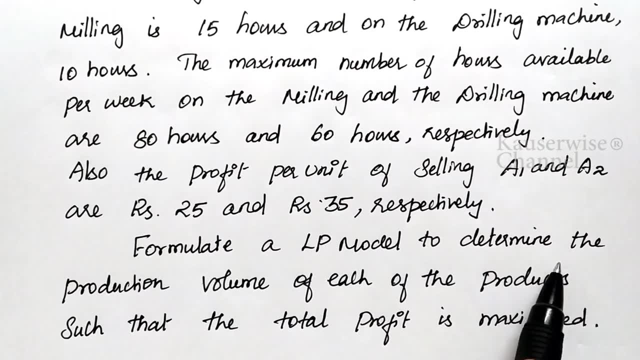 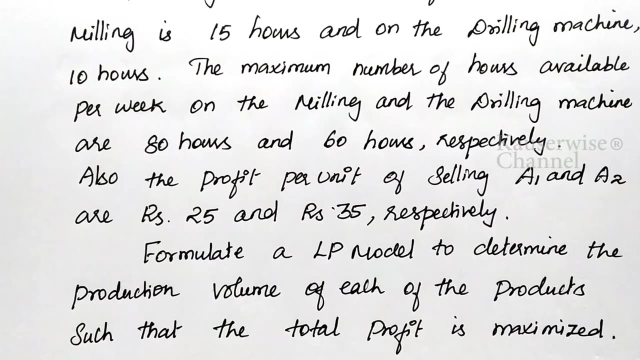 information given in the problem. Now, with this you can easily formulate LPP model. See, the question is: formulate a LPP model to determine the production volume- Okay, Production volume of each of the product. Here we have two different products, A1 and A2.. They ask you to determine. 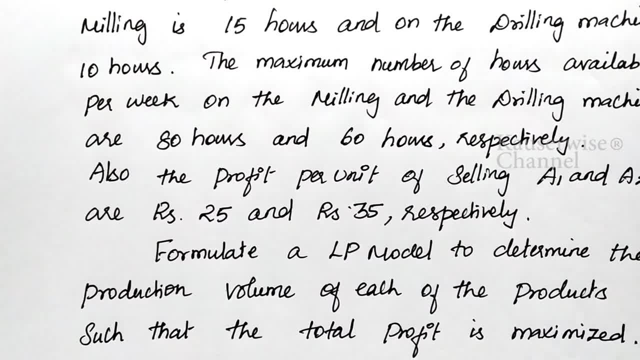 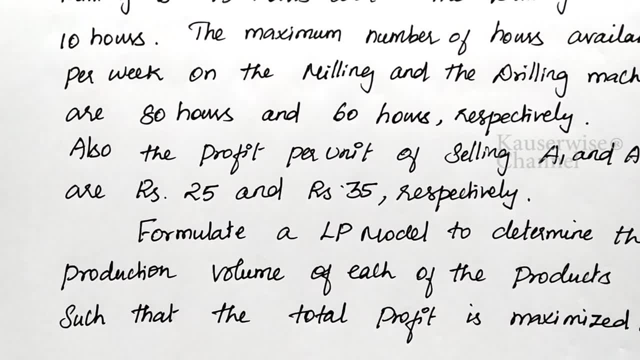 the production volume. So production volume of each of the product, So production volume of each of the product. So production volume means how many number of product you are going to produce, Okay, In order to maximize the profit, So that. So here we are going to use X1 and X2 for volume of. 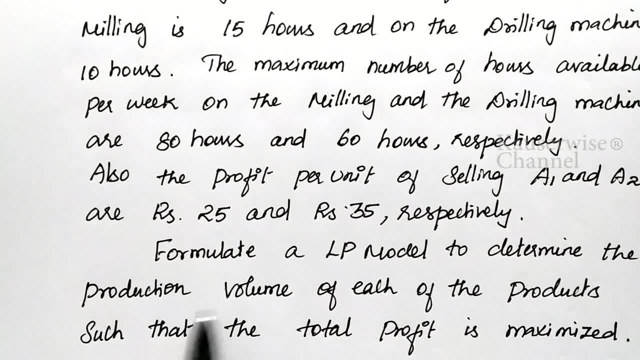 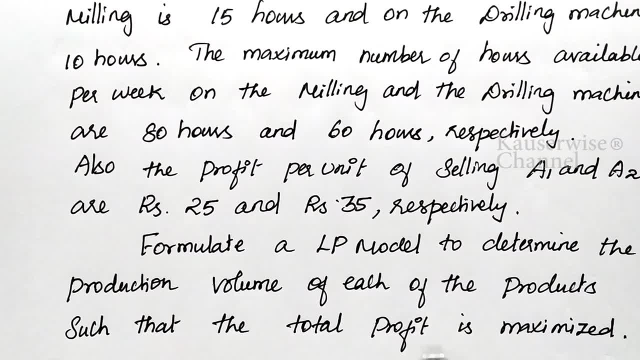 production, That is, number of product A1 and number of product A2.. In case, if we have three different products like A1, A2 and A3. Okay, Then we need to use X1, X2 and X3 for volume of production. Okay. 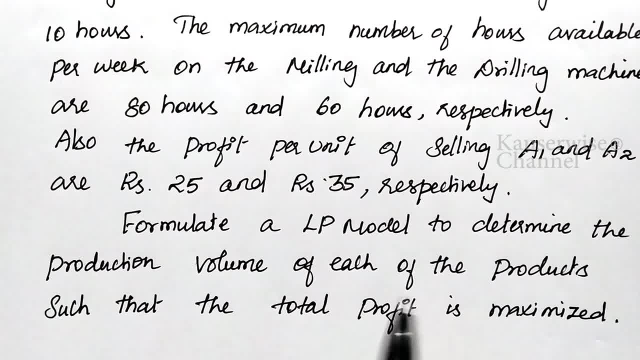 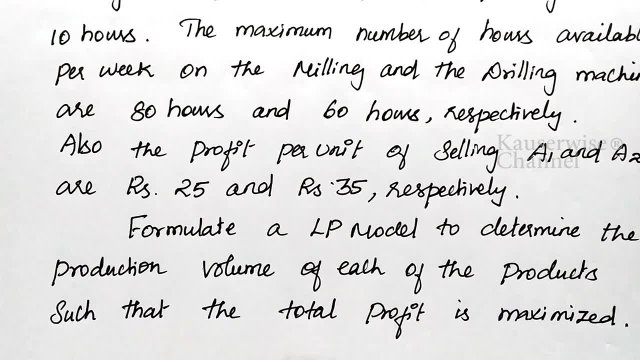 But in this problem, How many types of products are there? Two, That is, A1 and A2.. Okay, Here, let X1 and X2 be the volume of production. Okay, That is production volumes. based on that you can construct the LPP. 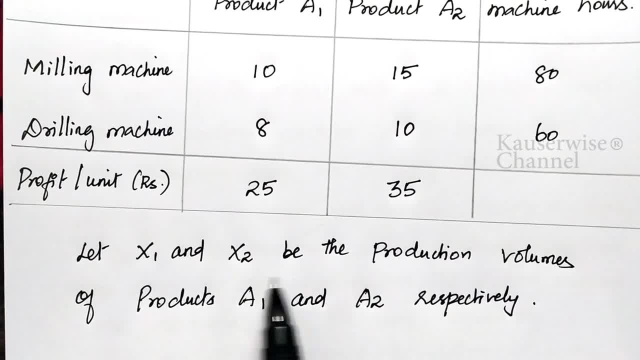 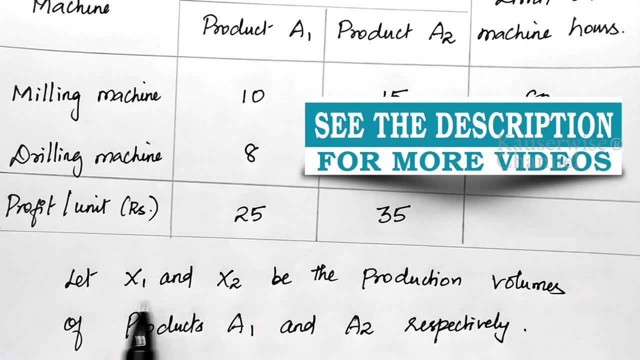 model: See: let X1 and X2 be the production volumes. Okay, We are going to find out how many number of A1 and how many number of A2.. So here we don't know X1 and X2.. This is a decision variable, Okay. 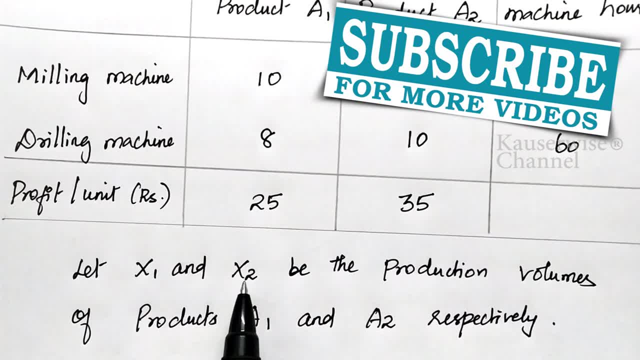 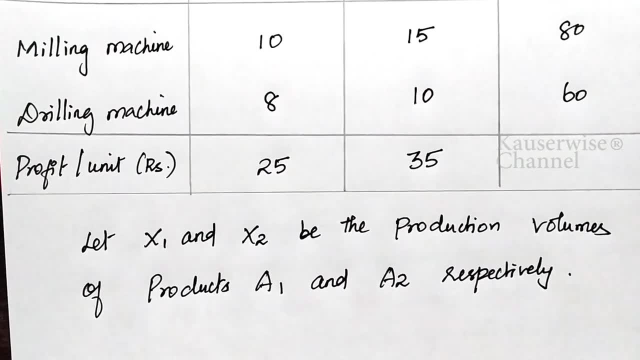 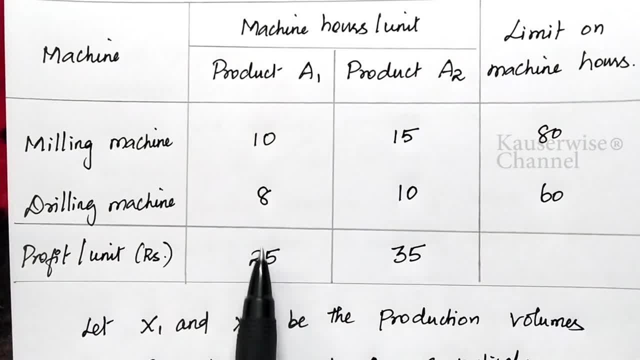 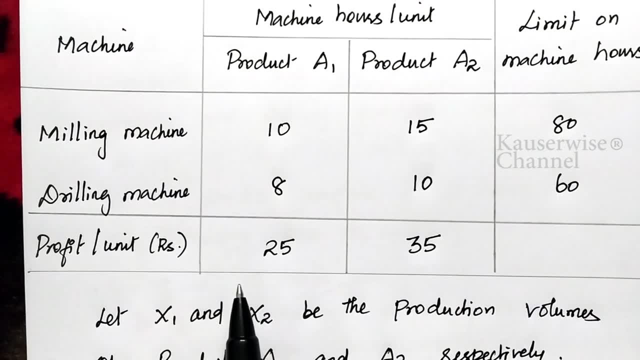 unit: 25 rupees per unit of A1 product and 35 rupees profit per unit of A2 product. We don't know how many number of product A1 can produce to gain maximum profit. In the same way, we don't know 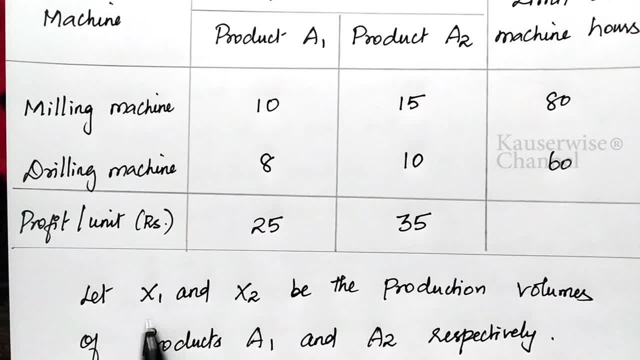 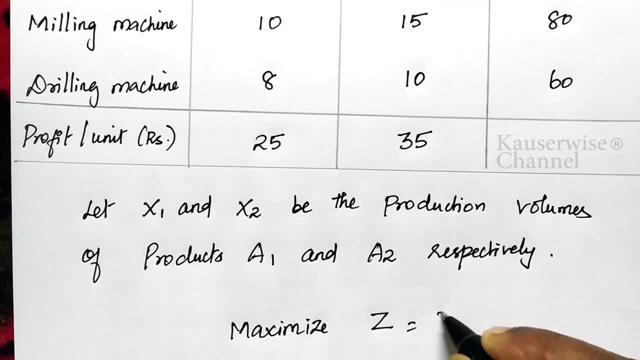 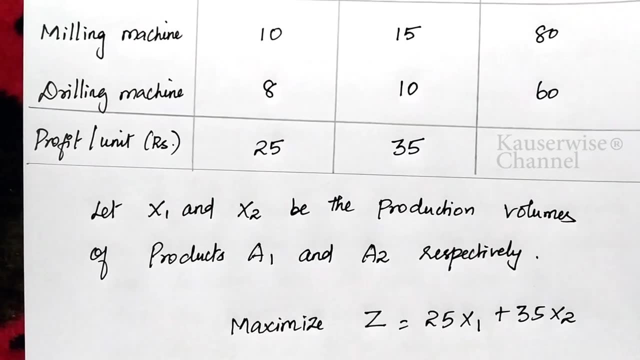 how many product we can produce so that we can maximize profit. So the product can be, the number of product can be X1 and X2.. So maximization Z is equal to 25 X1.. Okay, Plus 35 X2.. This is our. 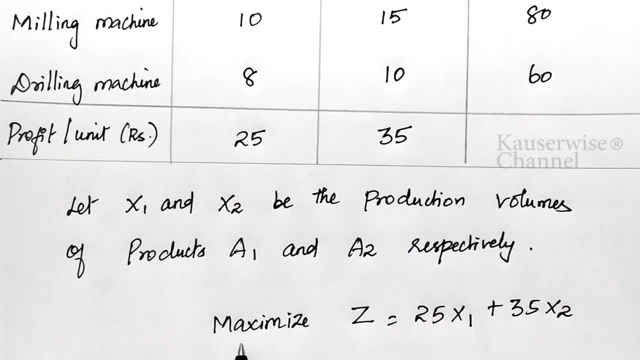 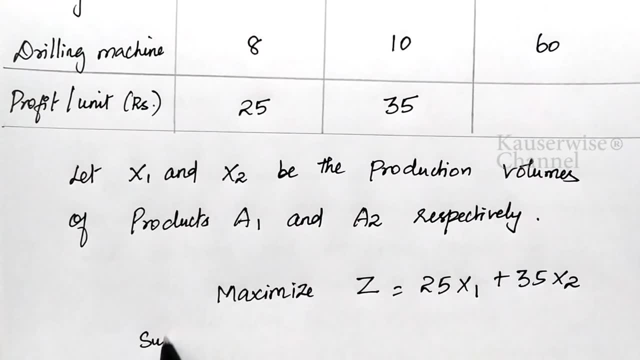 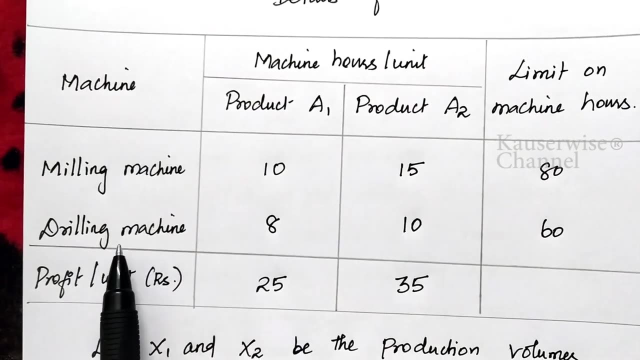 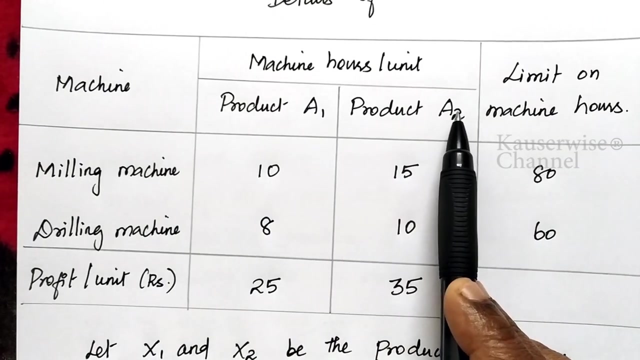 objective function. Okay, Our objective function is: maximize. Z is equal to 25 X1 plus 35 X2.. Okay, Subject to Subject to. Here we have two constraints. The first one is milling machine and the second one drilling machine. For milling machine for product A1.. Okay, 10 hours per unit is required For A2. 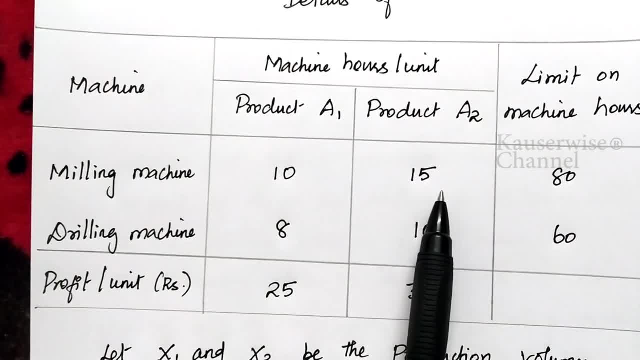 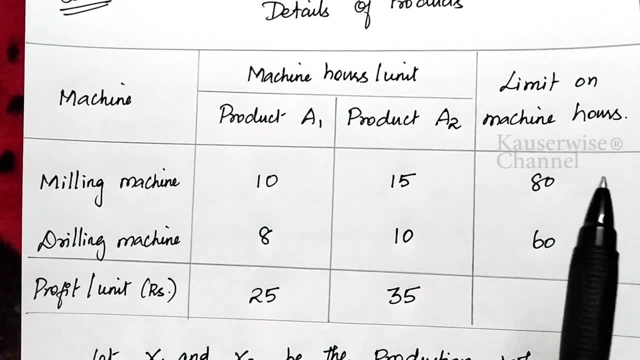 15 hours per unit. Okay, This is the constraint and subject to the limitation. See here. the limit is 80 hours You can use milling machine per week. How many hours? 80 hours. This is the available resource. So maximum you can use 80 hours. Okay. 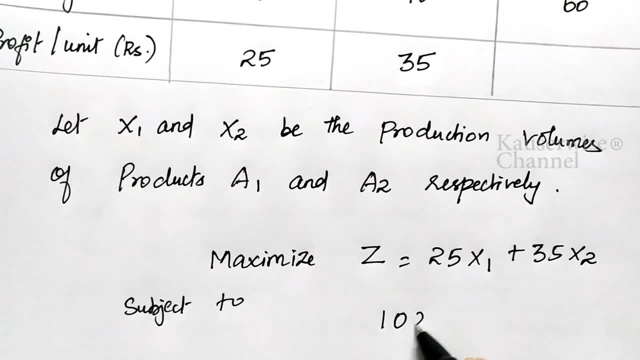 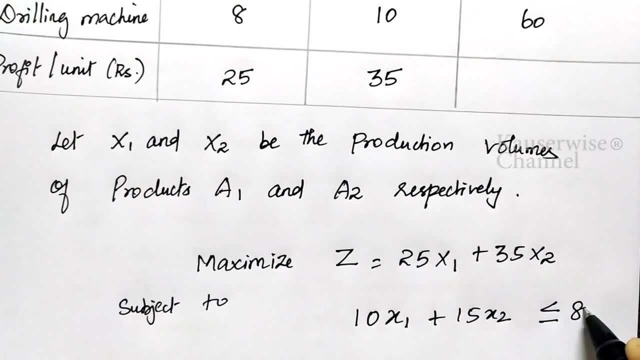 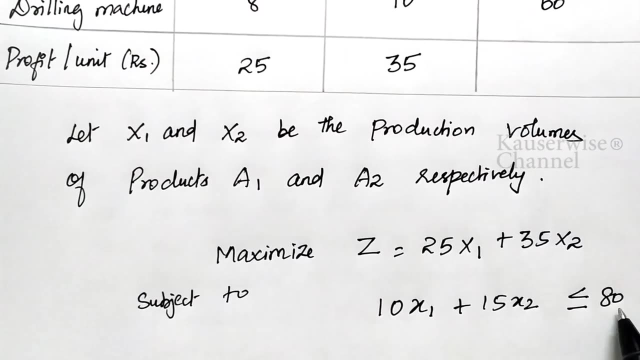 Okay, This constraint will be subject to 10 X1 plus 15 X2.. Okay, Lesser than or equal to 80.. Okay, Here, maximum 80.. No, So you can use 80 or less than 80.. So that lesser than or equal to 80.. The available. 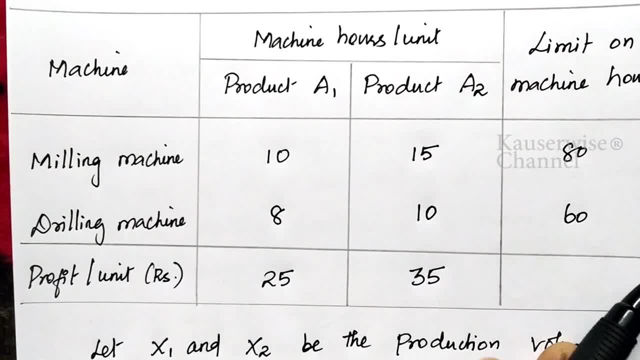 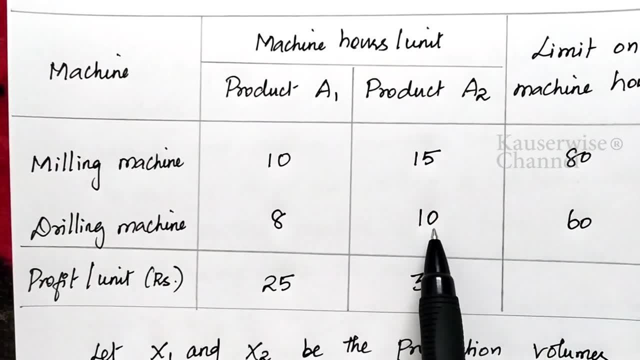 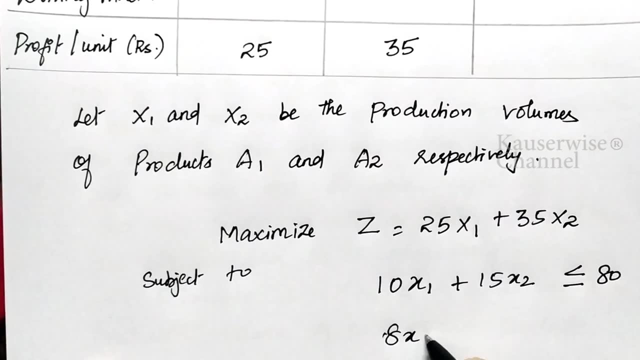 resource is only 80 hours per week- Okay. In the same way, in the second constraint, drilling machine for product A1- 8 hours and product A2- 10 hours- Okay, The maximum limit is 60 hours, Okay. The second constraint will be like this: 8 X1 plus 10 X2. 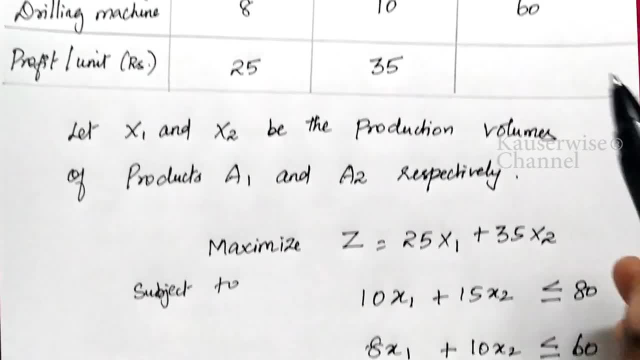 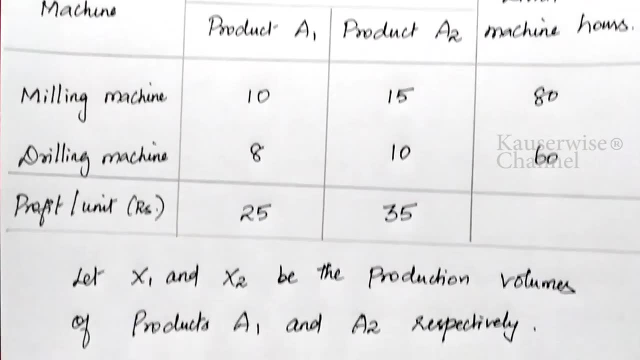 less than or equal to 60 hours, Because maximum duration is 60 hours per week, So that it will be 60 or less than 60. So that lesser than or equal to 60.. Okay, So this is the way to construct the. 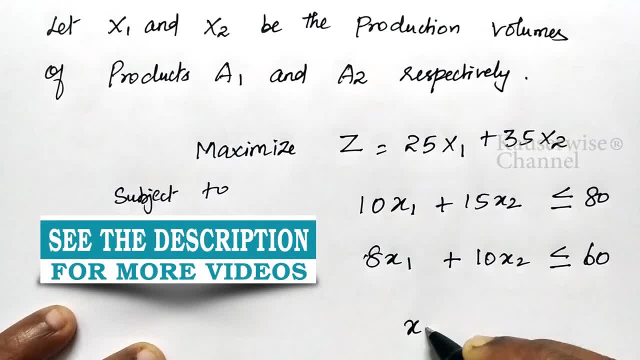 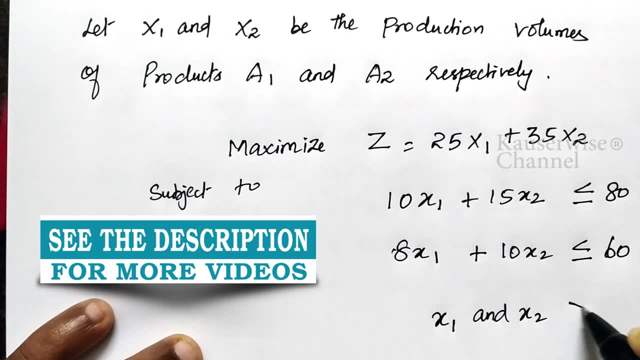 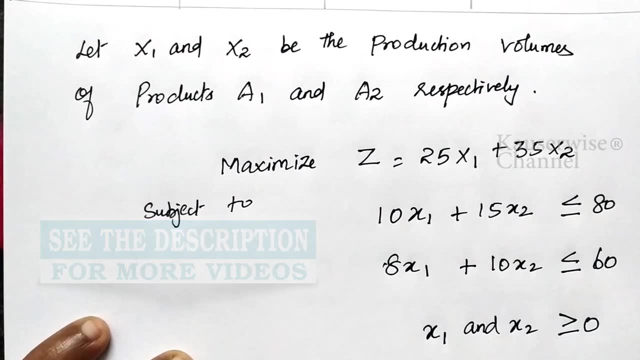 model and finally, you have to write like this: The final set of constraint will be, that is, X1 and x2 must be greater than or equal to zero. okay, so you are going to find out x1 and x2 value. no, in order to maximize the profit, so that the final x1 and x2 value must be non-negative constraints. 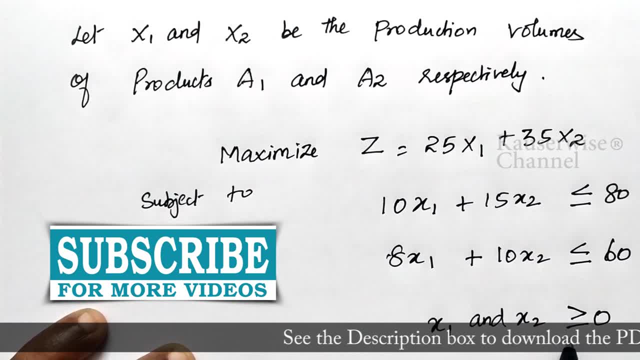 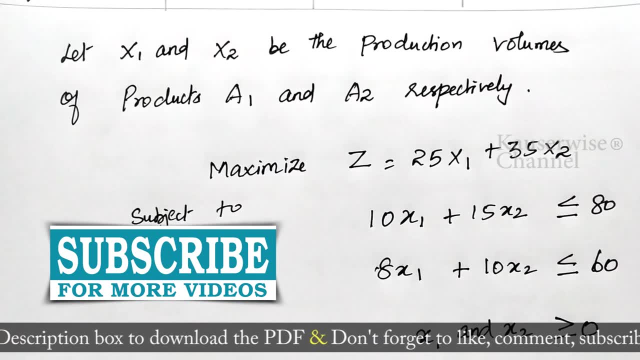 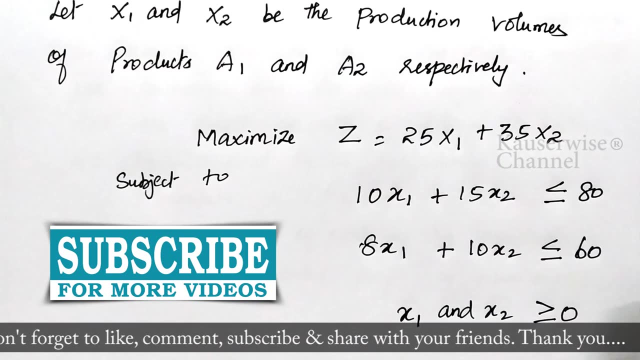 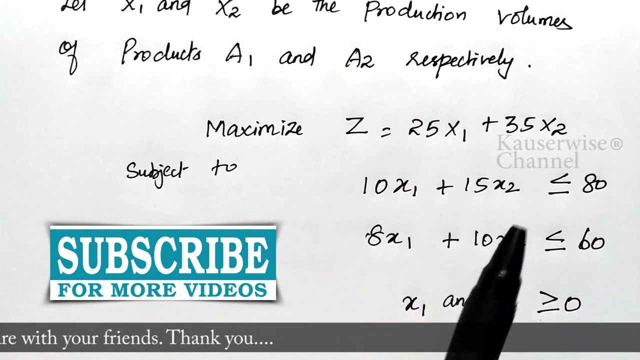 so non-negative means it should be positive, greater than or equal to zero, which means positive value only. so this is the way to construct or formulate or develop lpp model based on the problem. this is the model for maximization problem. okay, in the next video we will see formation of lpp model for minimization problem. you can find the playlist in the description. 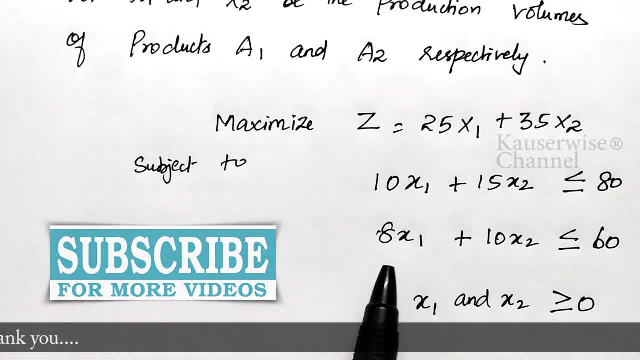 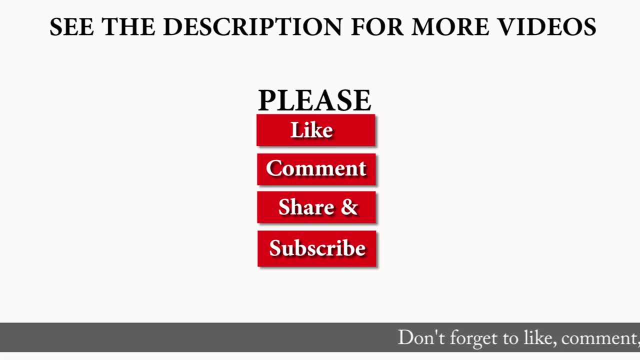 box. hope you like this video. please don't forget to hit the like, subscribe and share with your friends. thank you, you.